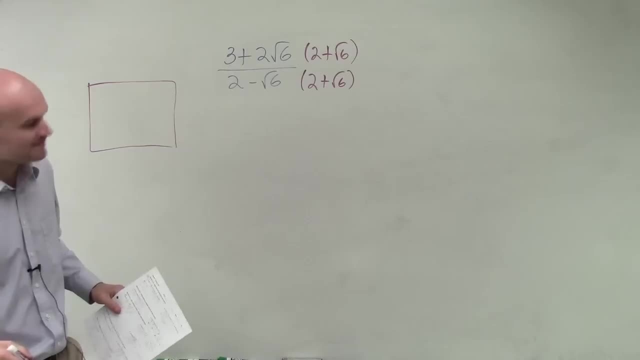 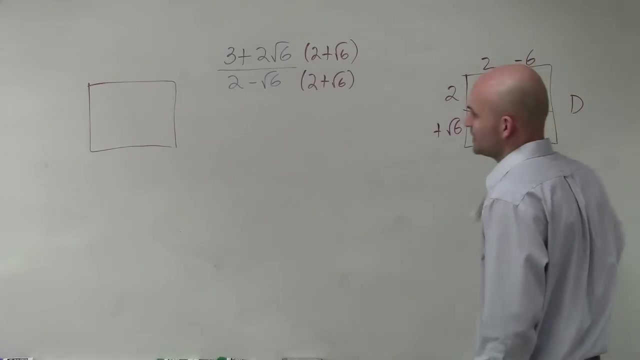 So I have to multiply my numerators and I have to multiply my denominators And again, I like using the box method, just to make sure everything is neat and in order. So this is the multiplication process for the denominator and this will be the multiplication process for the numerator. 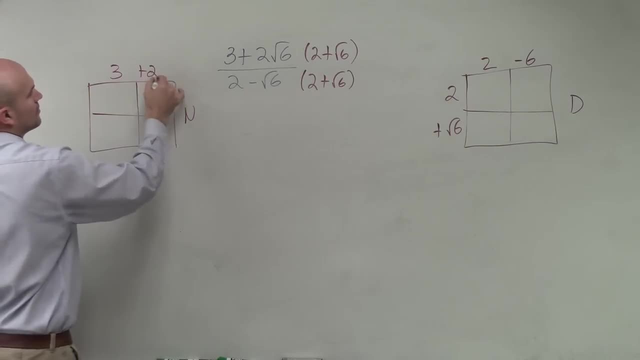 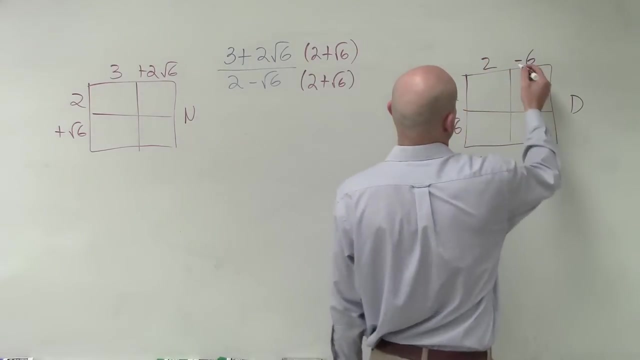 So all I do is I take both terms. Does everybody see how I have this set up? You have to multiply binomials in the numerator and in the denominator Square root of negative 6.. So now to use the box method. you just find the area of each box. 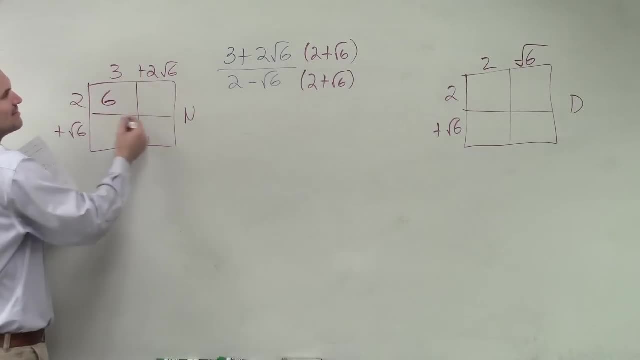 Length times width. 3 times 2 is 6.. 2 times 2. squared of 6 is 4 squared of 6.. 3 times squared of 6 is 3- radical 6.. Squared of 6 times 2 times squared of 6 is going to be 2 squared of 6 squared. 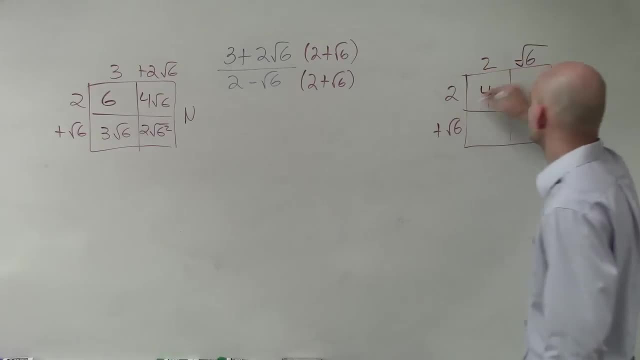 We'll simplify that in a second Over here: 2 times 2 is 4.. 2 times negative squared of 6 is 2 negative squared of 6.. 2 times positive squared of 6 is 2 squared of 6.. 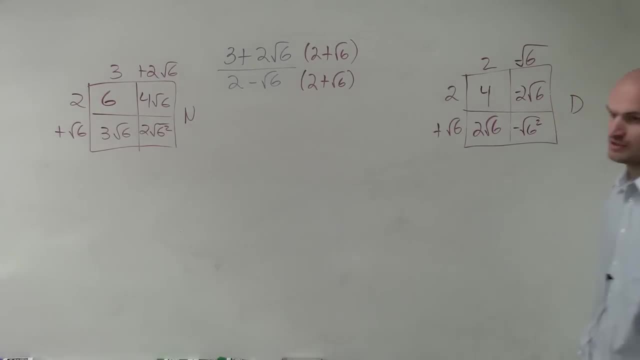 Squared of 6 times negative. squared of 6 is negative. squared of 6 squared. We'll simplify that in a second. Remember: this is your denominator and that's your numerator. Now let's write out our answer Now. remember: these two terms have the same radical. 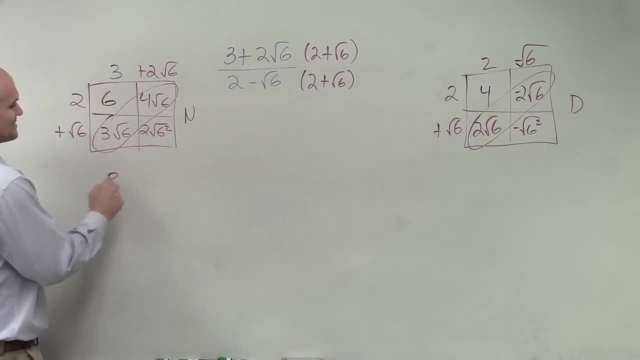 So therefore we can combine them. So I have 6.. 3 radical 6 plus 4 radical 6. It's going to be 7 radical 6.. Here, square root of 6 squared is just 6 times 2 is 12.. 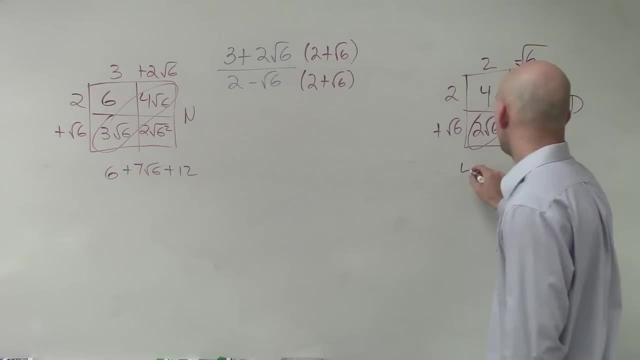 Right, And then over here I have 4. This becomes 0 square root of 6.. And then negative square root of 6 squared just becomes a negative 6.. So that's numerator or denominator. So let's simplify: 18 plus 7 square root of 6.. 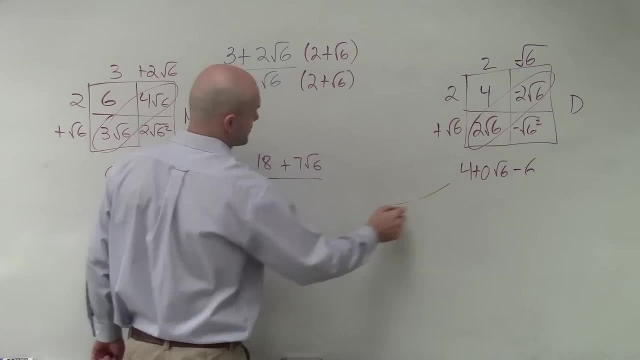 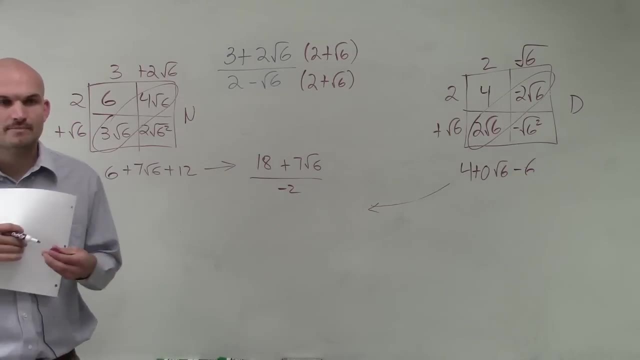 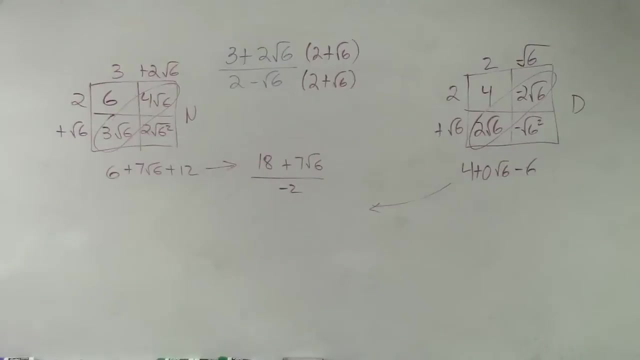 Which is your numerator, over the denominator which is negative, 2.. And that's it. Any questions on this? Okay, Then I'll do number 10..